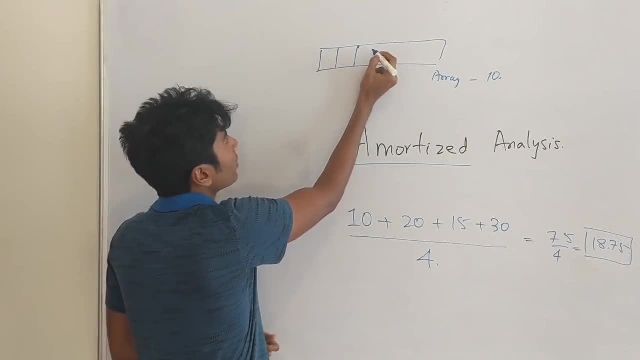 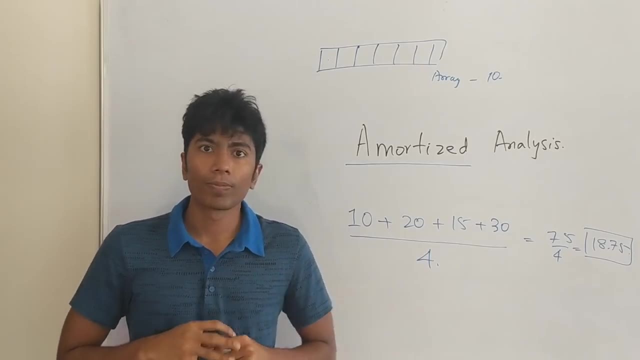 So you insert an array, Insert an element, Insert another element, So on and so forth, Up till you hit the maximum number of elements, which is 10.. Once you do that, what are you going to do? Well, the new element has to go somewhere. 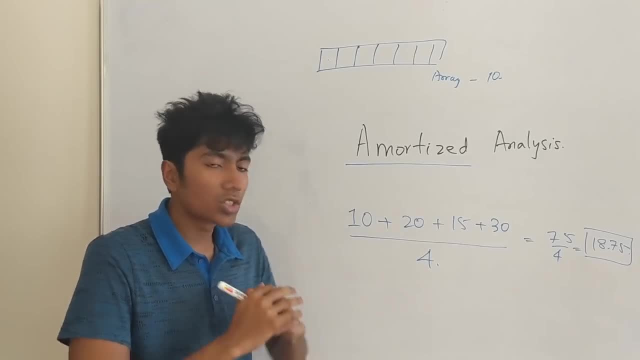 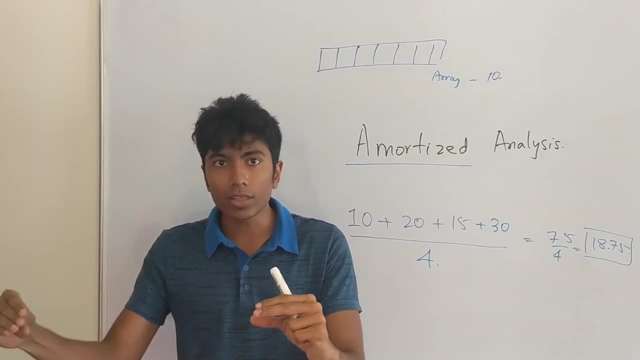 So one of the strategies that we can come up with is to just double the size of that array, And because arrays are fixed, they are actually locations in memory. You can't double the size of an array because maybe this part of memory is being used by the processor for something else. 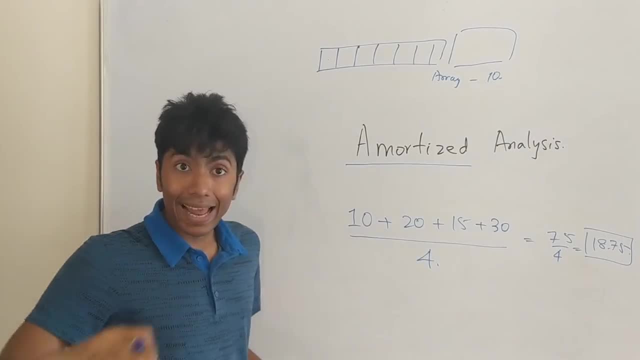 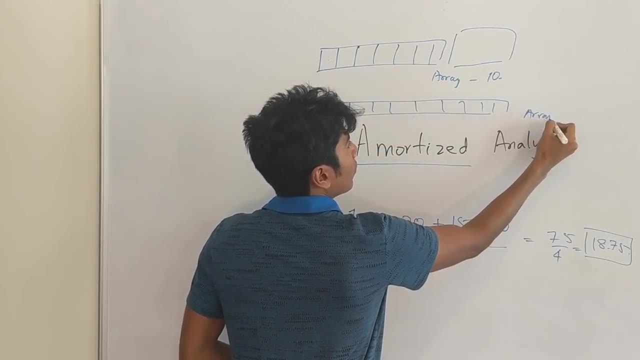 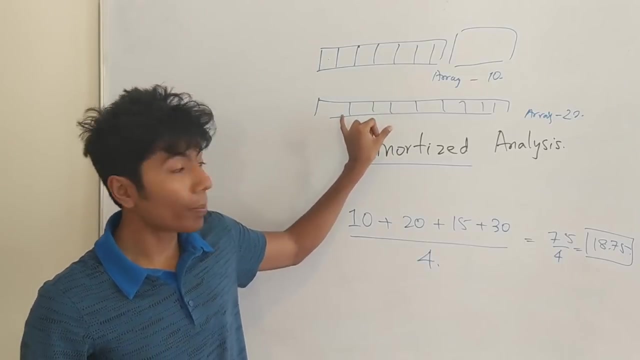 Okay, So here's what we are going to do: We are going to create an entirely new array of size 20.. The array size is now 20.. And we are going to take the first 10 elements from here and we are going to copy it over here. 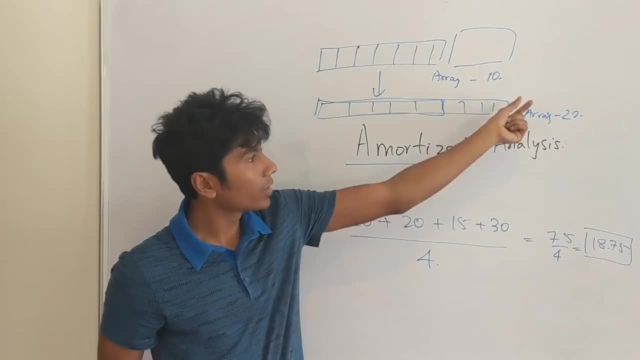 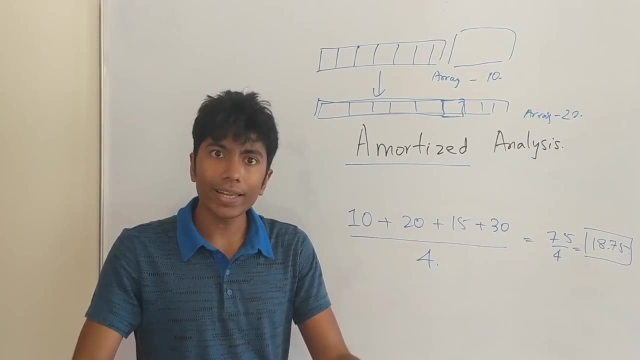 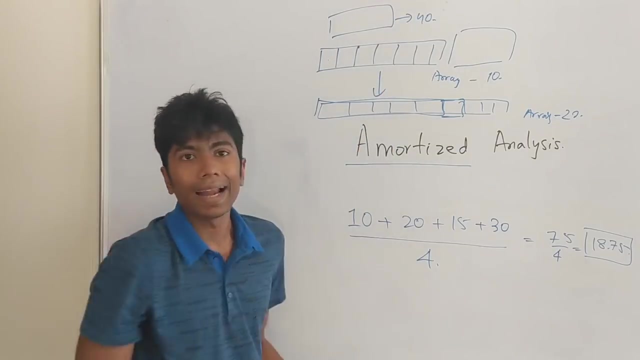 So that's one thing, And the new element, the 11th element, will come in here. Okay, Until you insert 20 elements. After that, you again double the size of the array to 40. And then to 80, and then to 160, and so on and so forth. 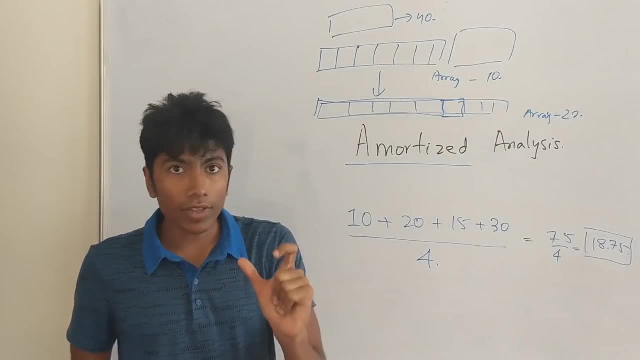 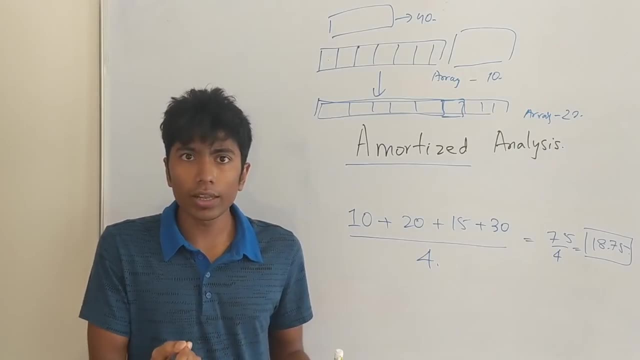 You see, what's happening here is that you are doubling the size of the array when you are hitting the maximum size of the array, And so what's happening is, every time you insert an element, there are either two things which are happening. One is you are easily able to insert the element. 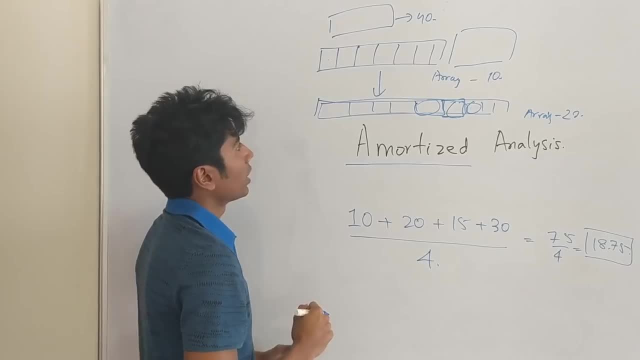 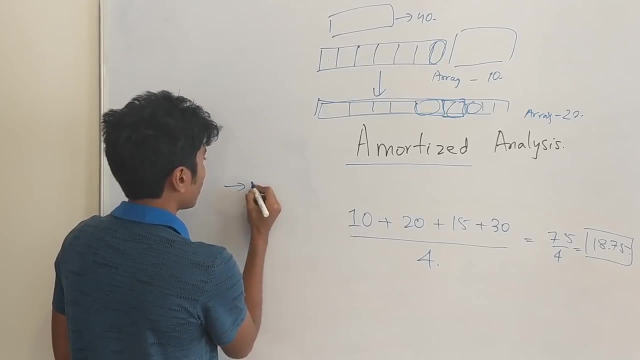 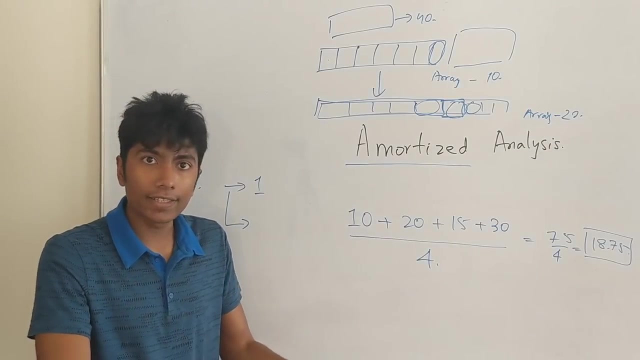 Especially if the element is over here or something. And if you are at the edge, then you have to double the size of the array. Okay, So cost of insertion is either 1 or it is the size of the array itself, Because what you are doing is you are doubling the size of the array. 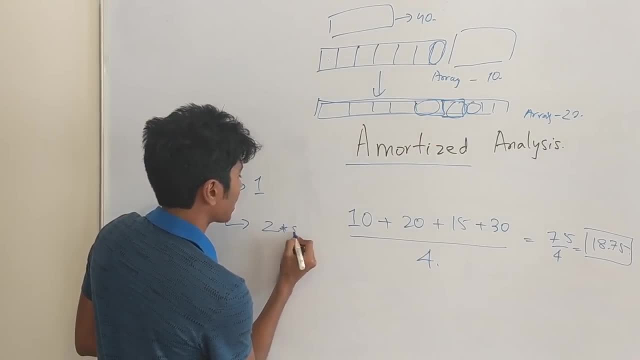 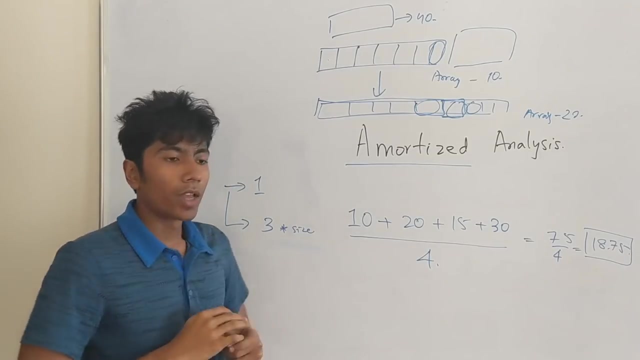 That is around 2 into size. Plus opting all the elements from here to here, That is again the size of the array itself. So overall this is 3 into size If you do the math. Okay, Now how are we going to analyze the complexity of this data structure? 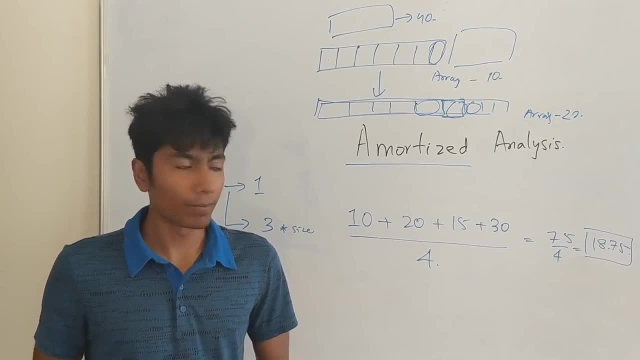 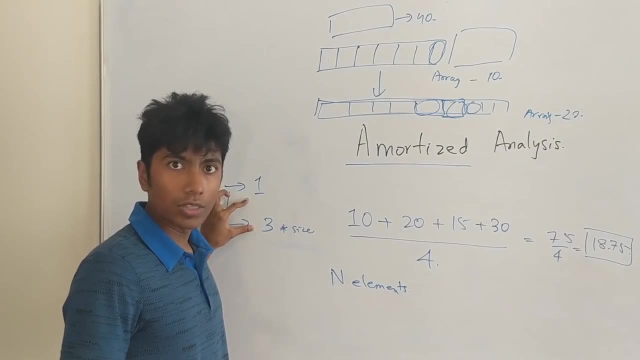 I am telling you that I am going to insert n elements into this array. Okay, These are the two variable costs that we have And we want to find out an advertised analysis of this. But first, before we get into advertised and everything, 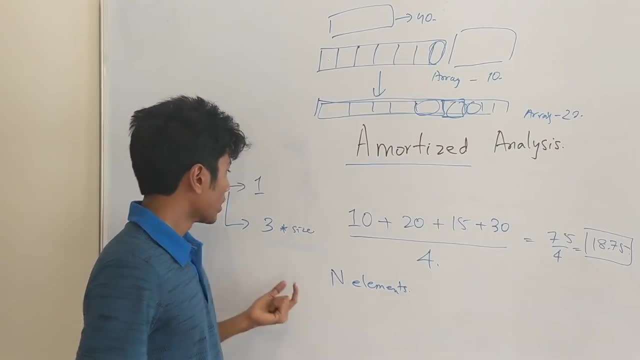 Let's go for simple analysis. The size of the array into 3 is the cost of every insertion. So in the worst case you have n elements For every operation. you are doing 3n operations And therefore n times your inserting elements. 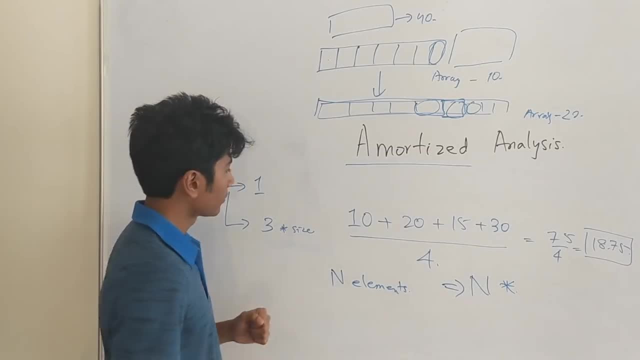 Each time it is taking you 3 into the size of the array. So that is 3n squared. Okay, That is the worst case complexity. I will just write it down here: Order n squared. This is one way to look at it. 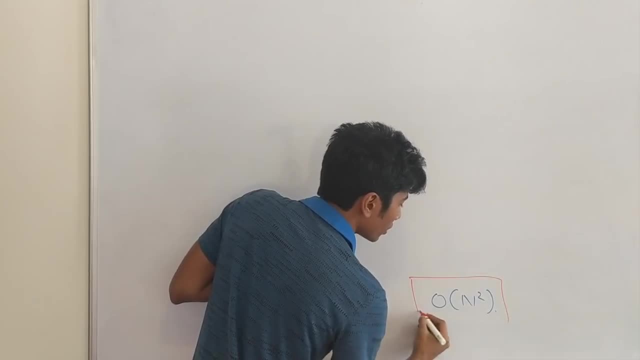 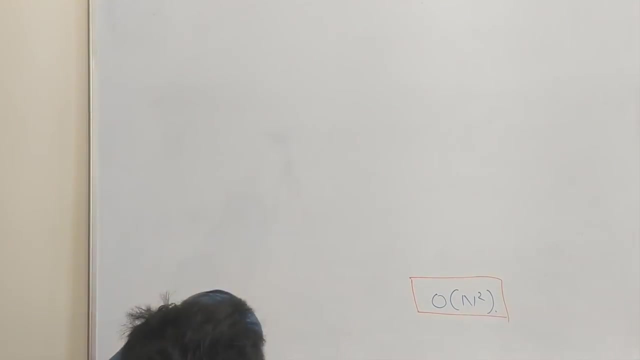 So, in the naive way to calculate things, We found order n squared To be the expected time complexity of n insertions. But this is This is a very pessimistic approach. What you can do is You can actually analyze it deeper. So let's say, initially I have the size of the array as 1.. So 1 insertion, No problem. For the second insertion, I have to actually double the size of the array. So let's take everything in account. 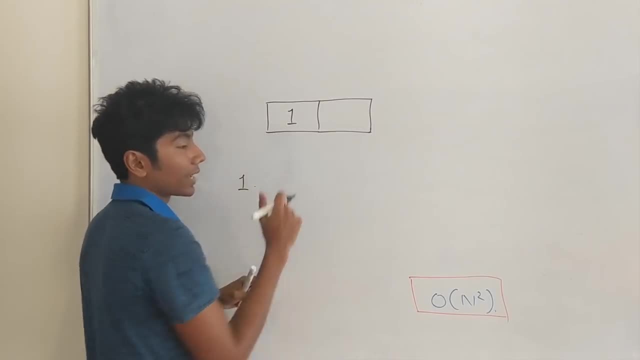 First time, insertion just cost 1.. Second time, the insertion has to double the size of the array, Plus I have to copy this element And then insert the new element, So that is Double the size of the array, which is 2.. 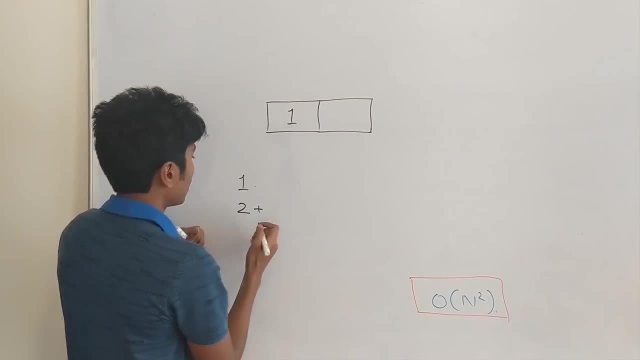 Plus. This is a new array. now, of course. Plus, copy the element which is 1.. Plus, insert the new element, which is 1.. So that gives me this new array, After which, if I need to add a new element Again, I have to double the size of the array, which is 4.. 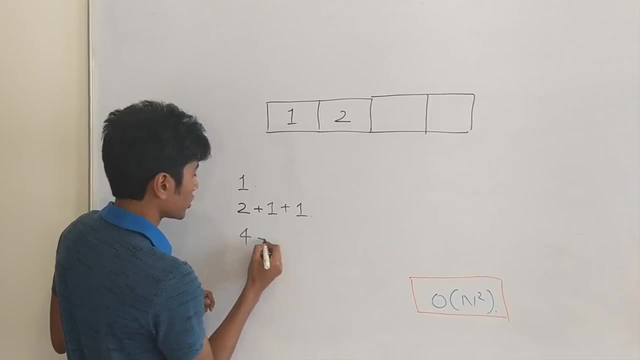 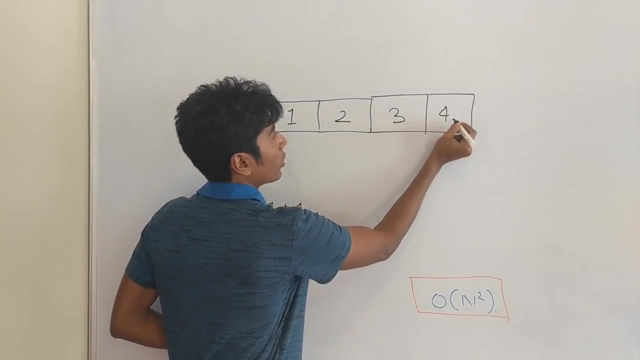 So that is 4 operations Plus. Copy the two elements And insert the new element, That is 3.. Now you will see the magic happening. The fourth element can just come in with one shot, That is 4. Again, 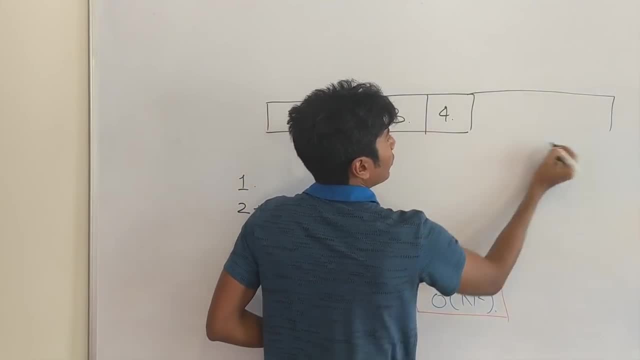 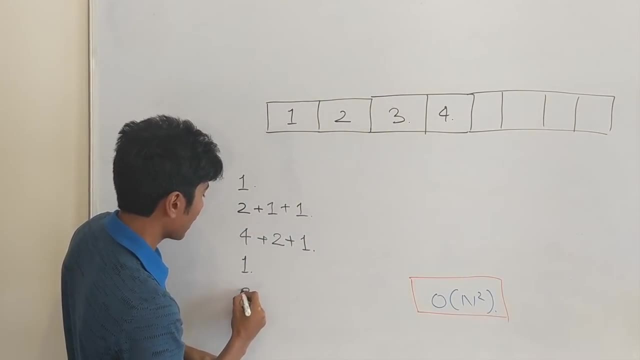 After 4, we need to double the size of the array For the new element. So that is this: And doubling the size of the array cost us 8.. Plus Copying the element, which is 4.. Plus Actually adding the new element, which is going to be the fifth element. 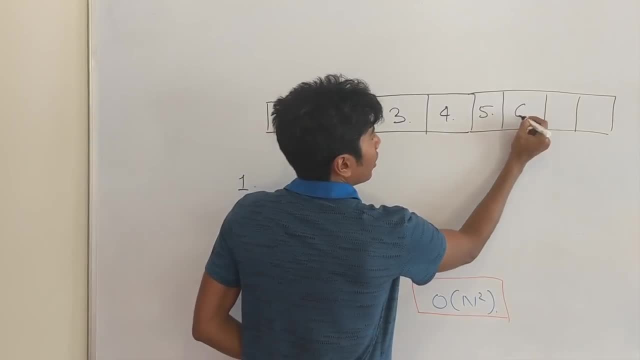 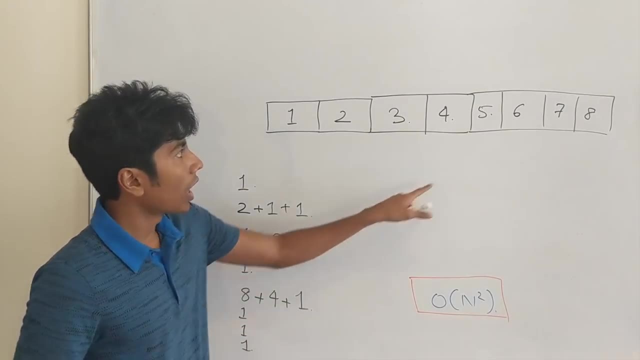 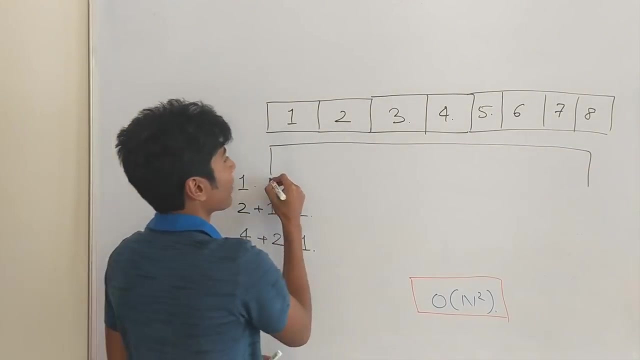 Now 6,, 7,, 8.. Just take one operation each And you are getting just over here After this when it comes to. So I am just going to draw it in the new line. But this is attached. It is the same array. 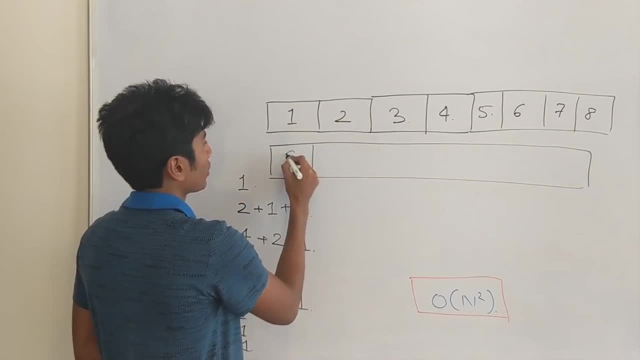 When a new element, 9, comes in, The cost is actually creating a size which is double, Which is 16.. Plus copying the old 8 elements into the new array Which is going to be somewhere over here. So plus 8.. 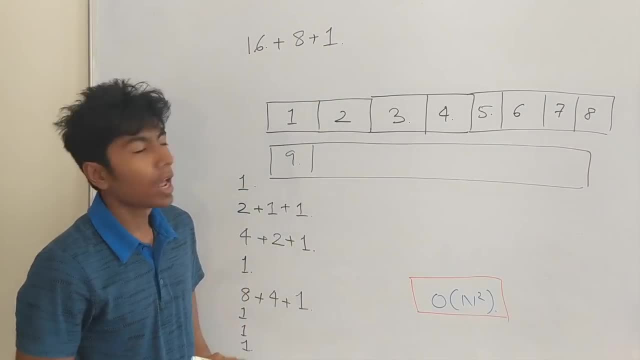 Plus the 9th element being inserted, which is 1.. And then you have 10 levels of the array. So you have 10,, 11,, 12,, 13,, 14,, 15,, 16.. All of them taking just one operation. 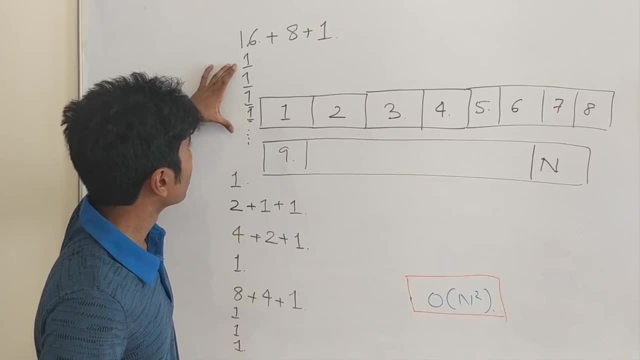 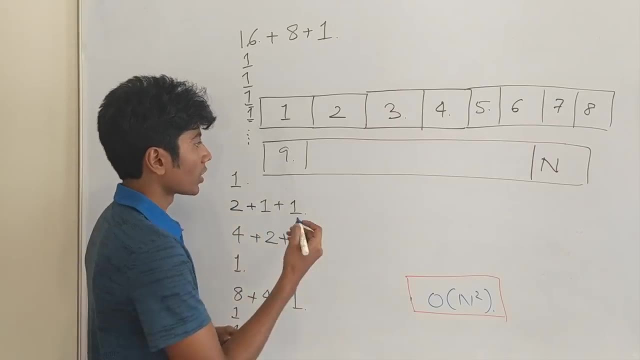 And this is useful information, Because you are doing the cheaper operations far more frequently than the expensive ones- And how many times are you actually doing the expensive ones? The first time, the array size is 1.. The second time, when you are doubling, the array size becomes 2.. 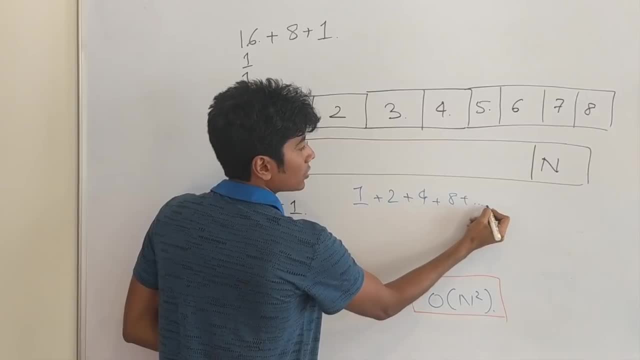 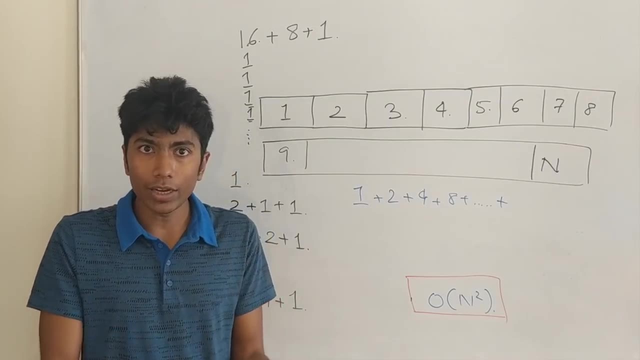 Then it becomes 4.. Then it becomes 8.. Then it becomes 16. And so on and so forth. Up till what size In the worst case? the number of elements that you have That you are going to be inserting. 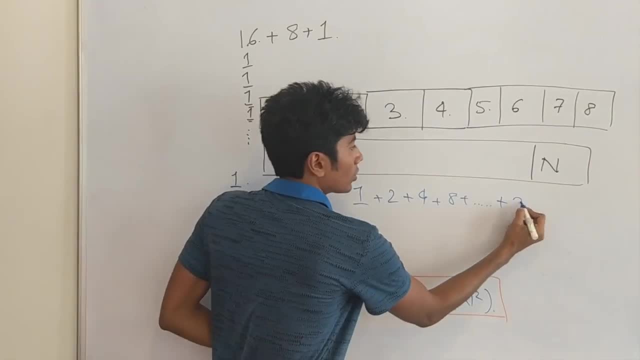 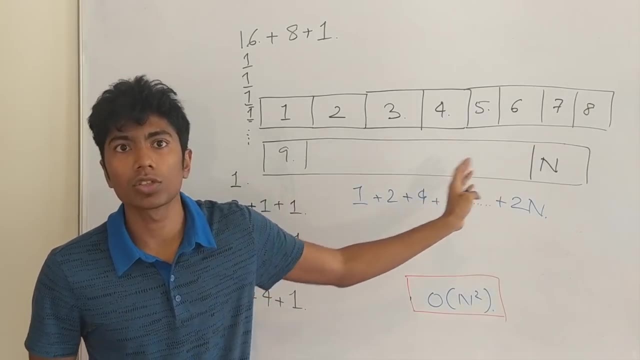 Is around half of the size of the array, So up to 2N. Why is that? Because when you have inserted all your elements, The only extra space you can have is almost double, Because you are doubling the size of the array. 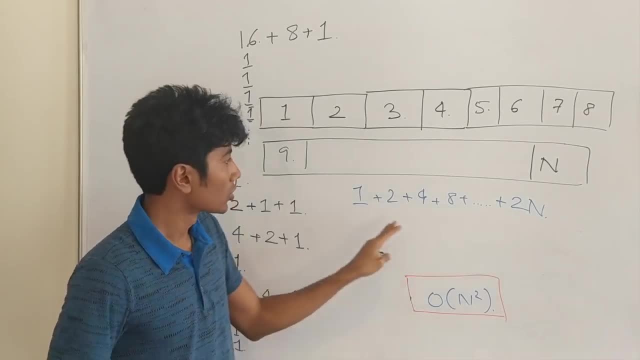 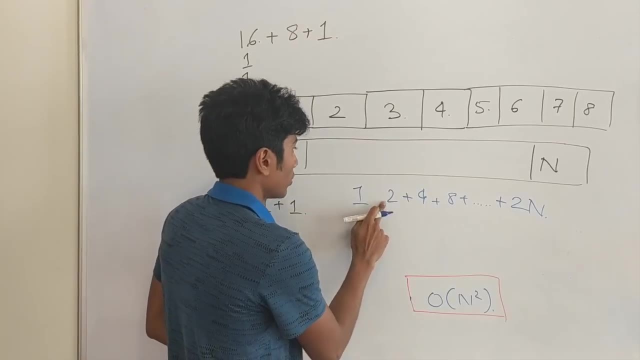 So the maximum size you have hit is 2N at most. So from 1 to 2 to 4 to 8, up to 2N Is the size of the array, The shifts in the size of the array. 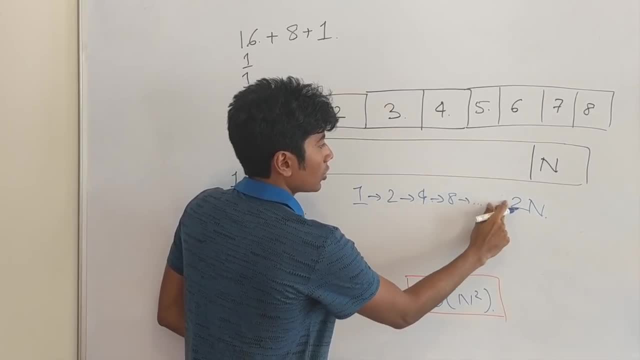 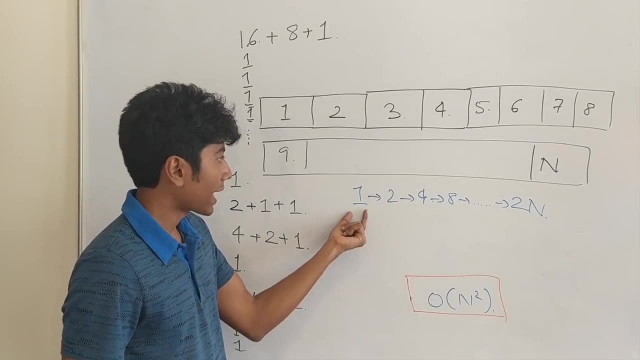 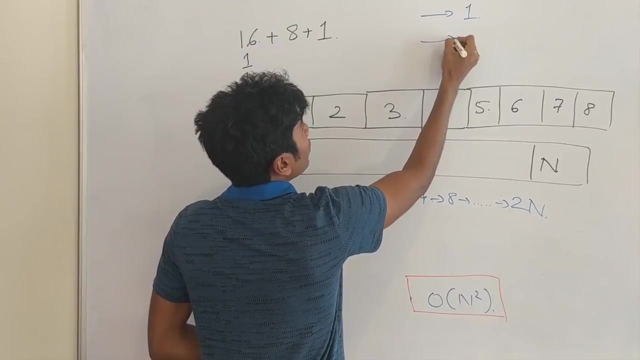 Okay. So this is interesting Because every time you are doing this, You are doing 3 times the size of the array cost, Which is Every time you are doing either just one operation Over here Or you are doing 3 into the current size. 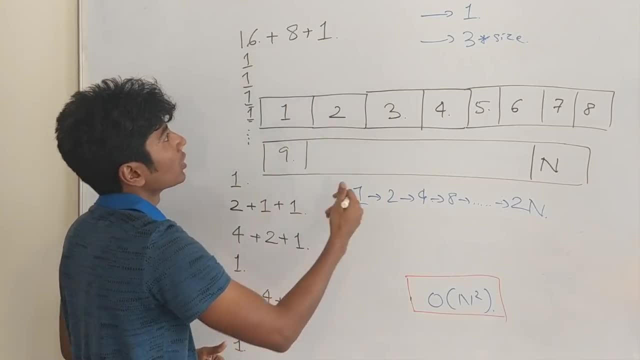 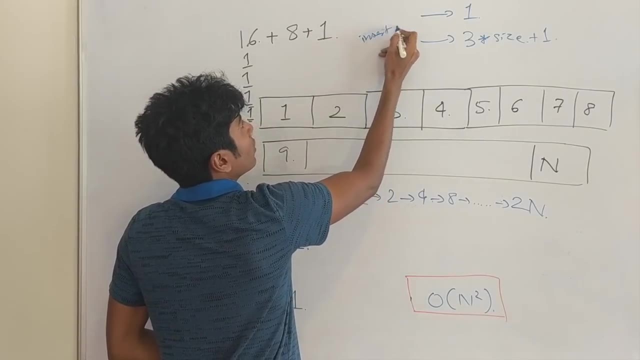 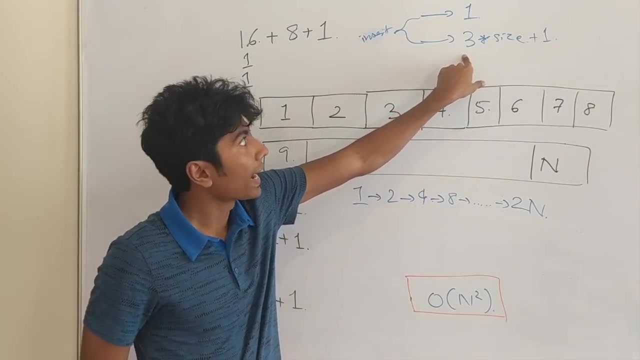 Which is over here, 24 plus 1.. 3 into the current size, plus 1. actually, That is an insertion. Okay. So for all of these, What we are going to do is We are just going to multiply this by 3.. 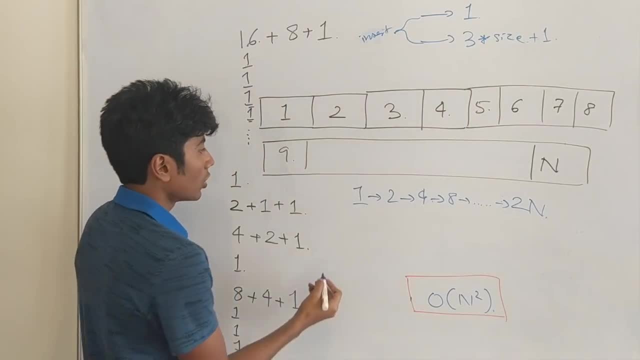 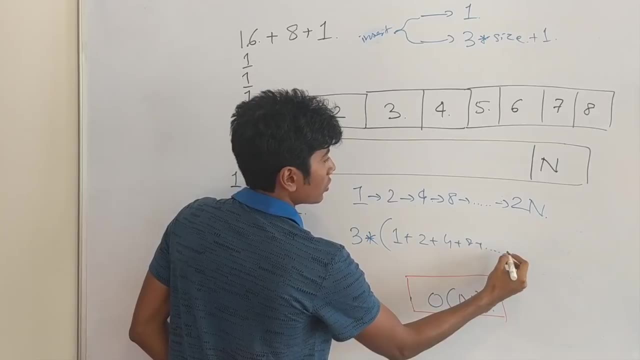 And add 1 to the number of times these operations occur. So all I need to do is just multiply this by 3.. Add them all up: 4 plus 8 plus 4, and so forth, Up to 2N. 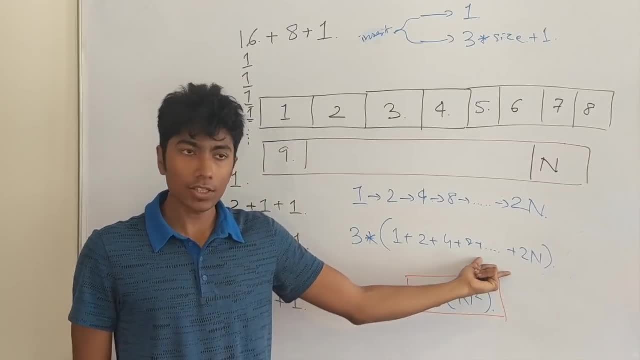 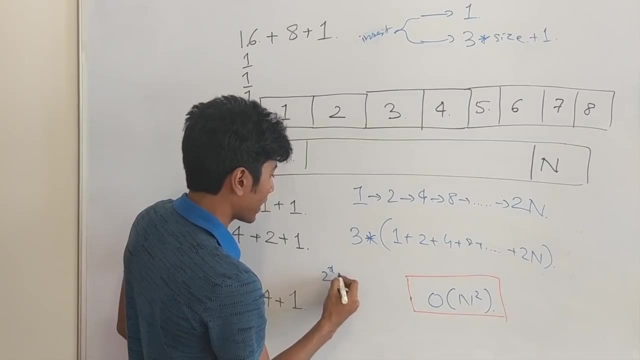 And how many times do I need to? What is the size of this series? From 1 to 2N, It turns out. This is a dramatic progression. 2 raised to the power of x is equal to 2N. That is because it is doubling the size. 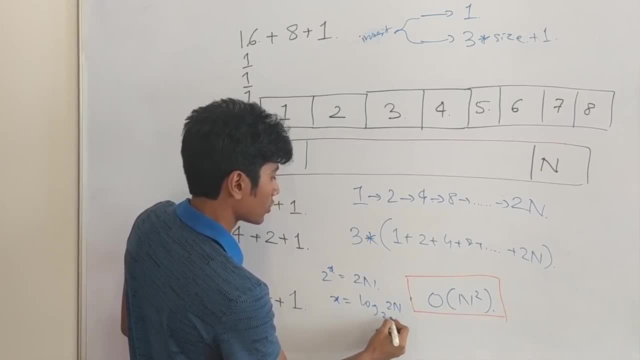 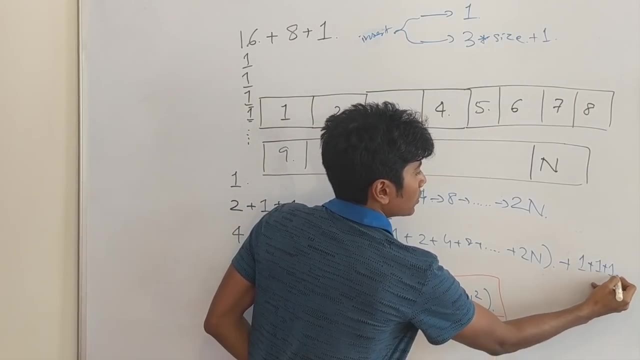 So x comes out to be log 2N, V is 2.. Okay, So this is just plus 1 plus 1 plus so on and so forth. Because of this extra term over there, This occurs Log 2N times. 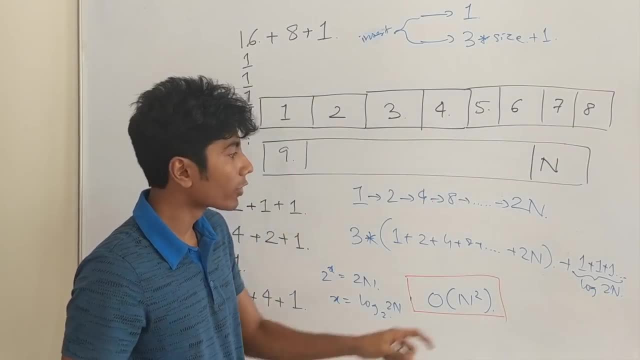 Okay, If you don't understand log N, Then you can have a look at the video, The previous video. I will have a link up there on the description below. But yeah, This is. This is really really small, So it can be. 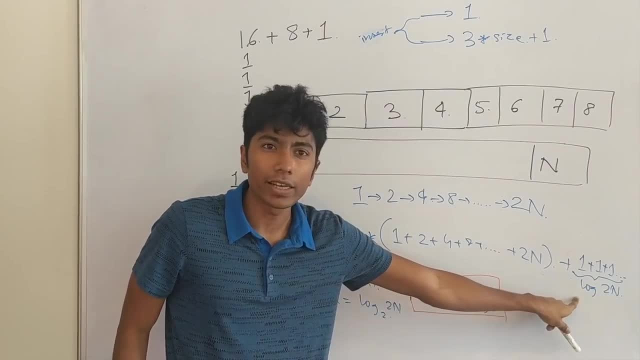 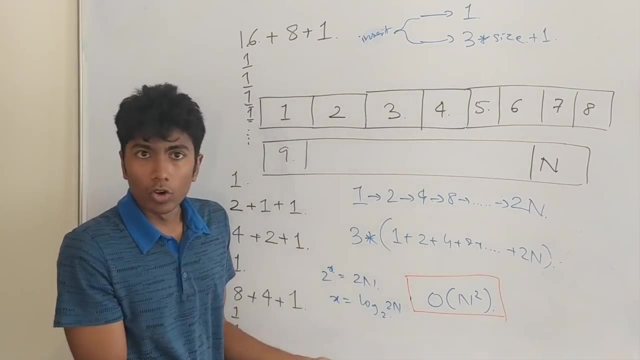 Ignored, Okay. On the other hand, This can't be ignored, Of course. This sum Is again a geometric progression sum, So 2N plus From 1 to 2N. This can't be ignored Because 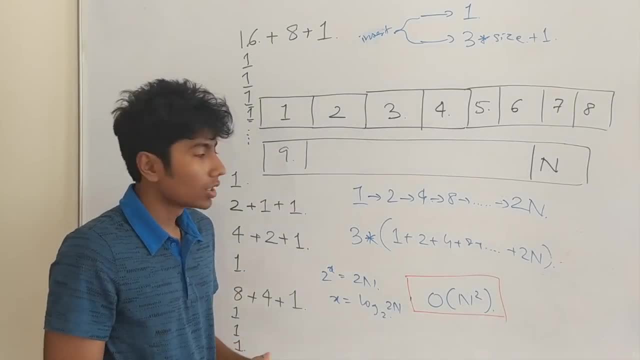 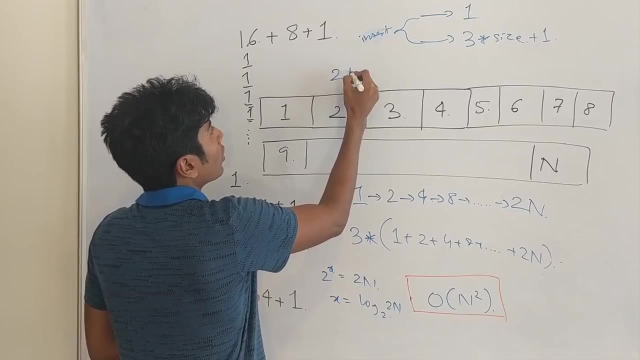 This sum Is again a geometric progression Sum, So 2N plus From 1 to 2N. This can't be ignored. Okay, The cost is 2N into 2. Minus 1. Okay, 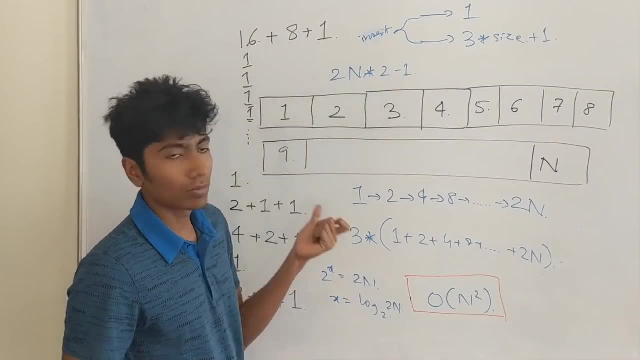 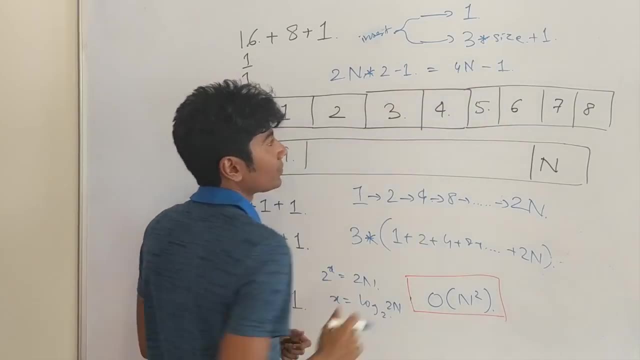 This is just a Geometric progression sum. Just Take my word for it. This turns out to be 4N Minus 1.. Okay, And Multiplied by 3. Because the multiplication of 3 is over here. 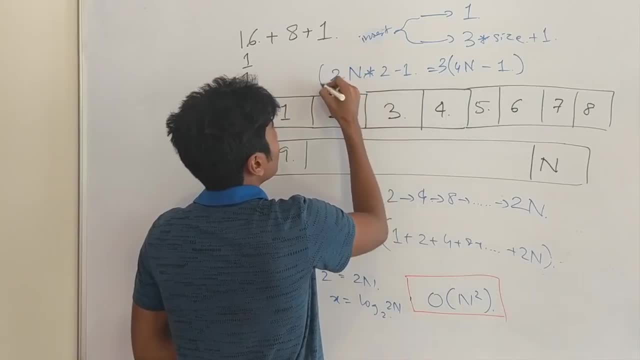 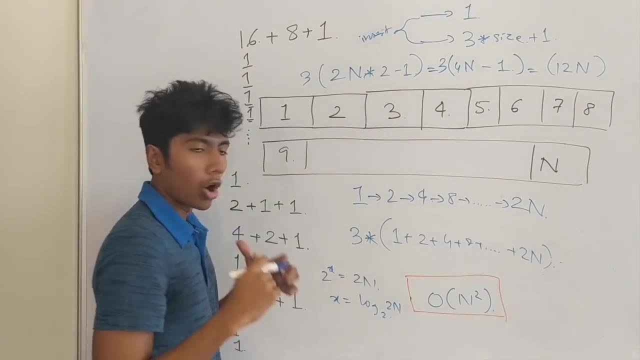 This turns out to be 12N. Right Order: Complexity Order: 12N The 12. N Is Over here, Right, So This 12N The 12. Is a constant.